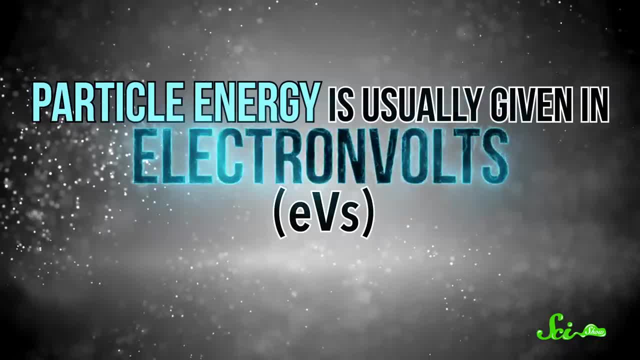 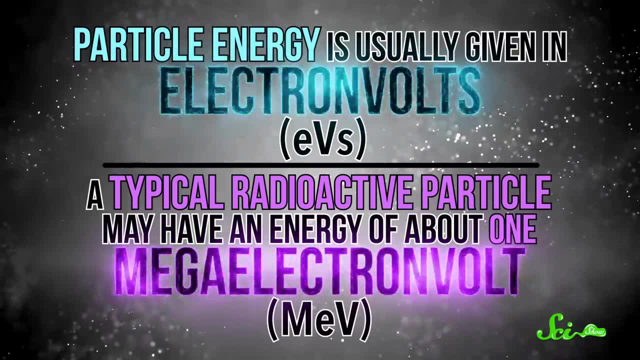 So that's where we get to our first radiation units. Particle energy is usually given in units called electron volts or EVs, And a typical radioactive particle may have an energy of about one mega-electron volt or MeV, That's a million EVs. 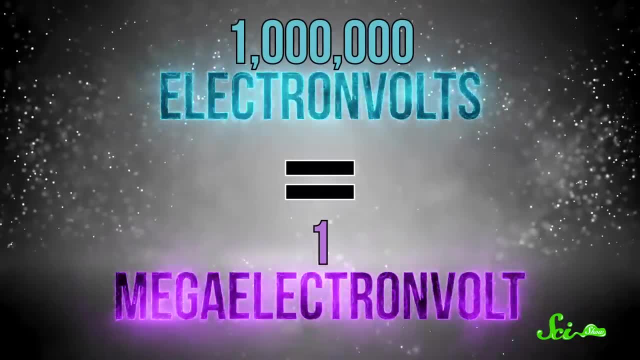 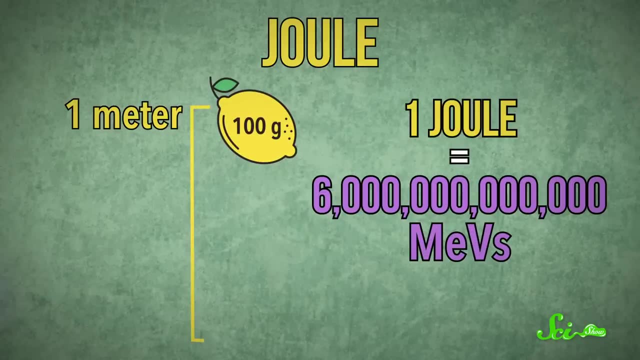 And while that might sound like a lot, it's nothing compared to our everyday standard unit of energy, the joule, The energy needed to lift 100 grams up by one meter, which has six trillion MeVs in it. So one particle has a tiny amount of energy on a human scale. 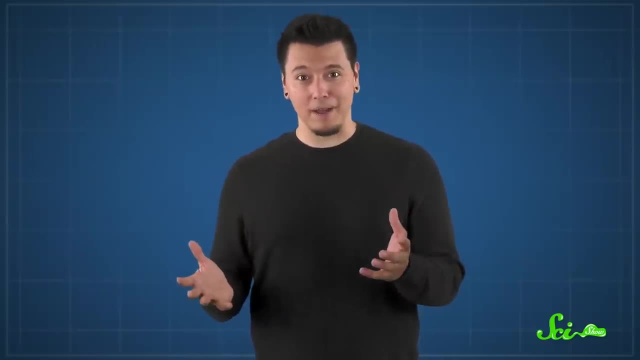 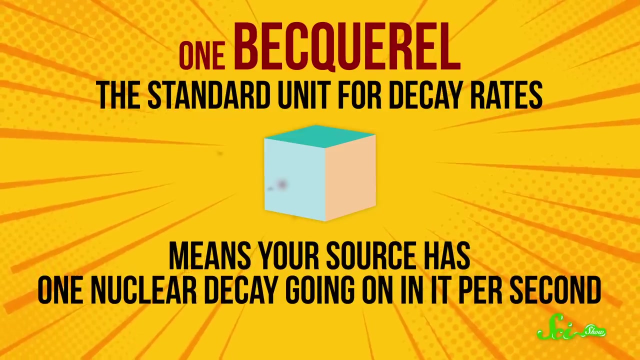 Of course radioactive sources don't generally give off one particle at a time, So we also have units to describe how many radioactive decays happen in a source per unit. So that's the first one source per unit of time. One becquerel—the standard unit for decay rates—means your source has one nuclear 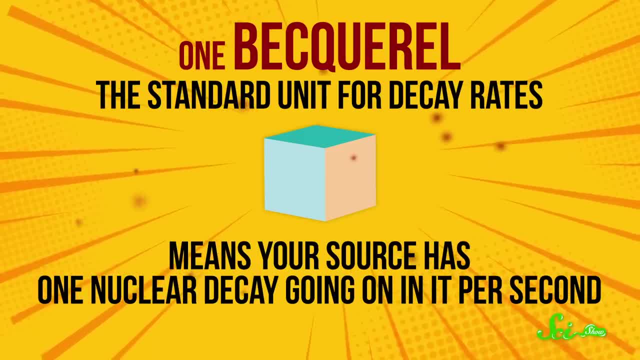 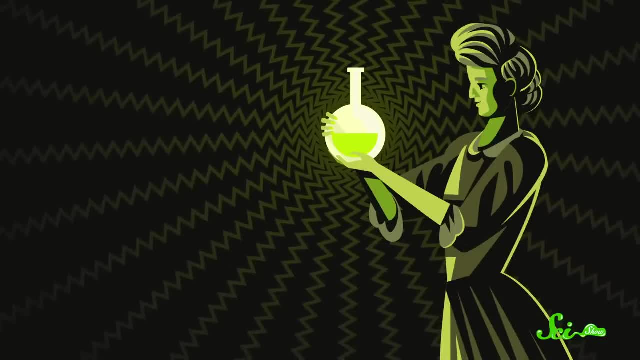 decay going on in it. per second—basically a tiny amount of activity- Your body typically and safely emits several thousand becquerels all the time. There are older units that describe decay rates too. The Curie, for example, was based on the decay of radium-226, but it's now defined as 37. 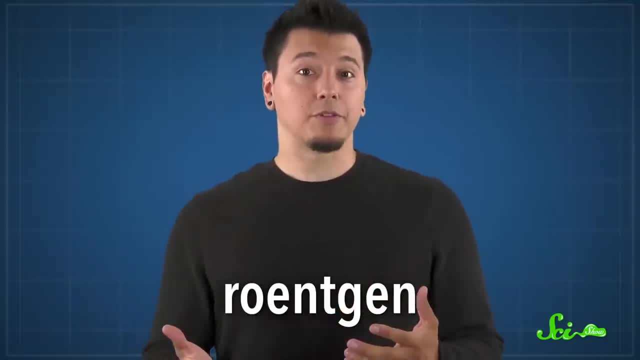 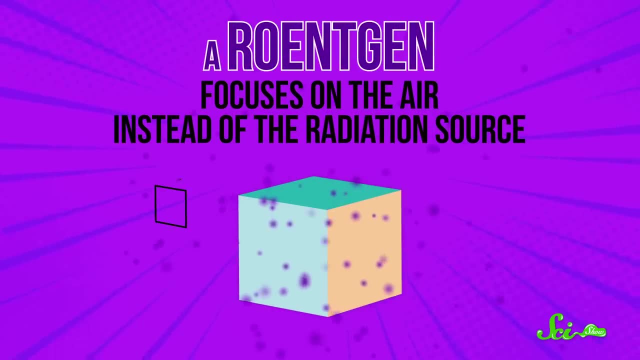 billion becquerels. Somewhat related is the Röntgen, which was in fashion for a while and recently popularized by the Chernobyl miniseries on HBO. It focuses on the air instead of the radiation source. Essentially, it quantifies how many electrons are being knocked off per cubic centimeter. 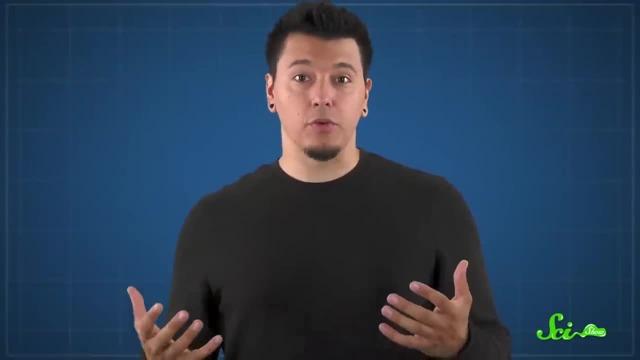 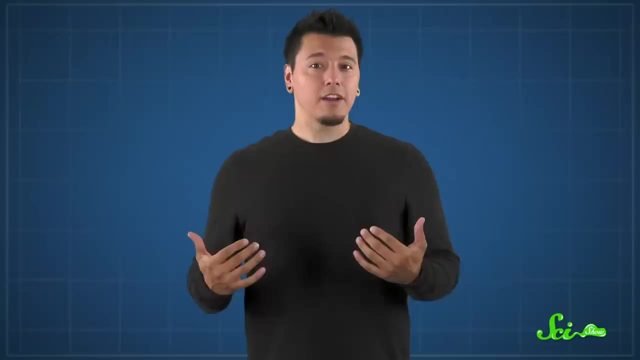 of air, And if you're standing next to something emitting one Curie of radiation, or in a room where a whole lot of electrons are being knocked off of air molecules, that's probably not great for you. But from a medical perspective it's not enough to know how many particles of radiation. 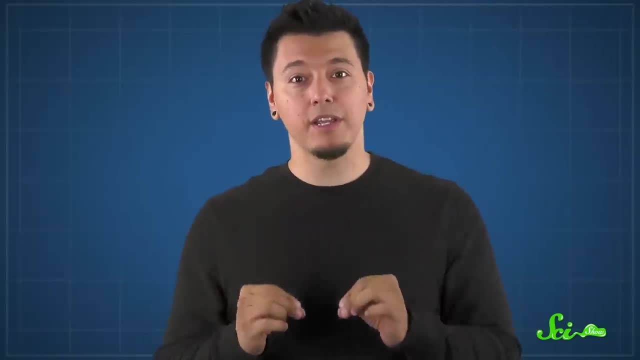 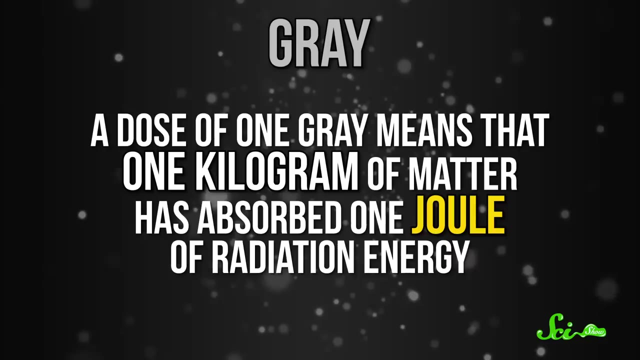 are in a room or being emitted by something, You need to know exactly how much radiation your body is absorbing. This is called the absorbed dose. The standard unit for the absorbed radiation dose is the gram. A dose of one gray means that one kilogram of matter has absorbed one joule of radiation. 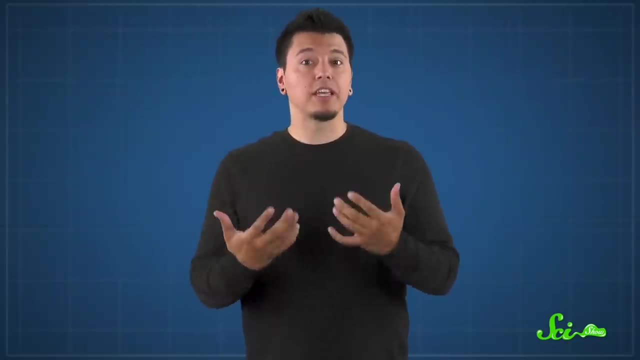 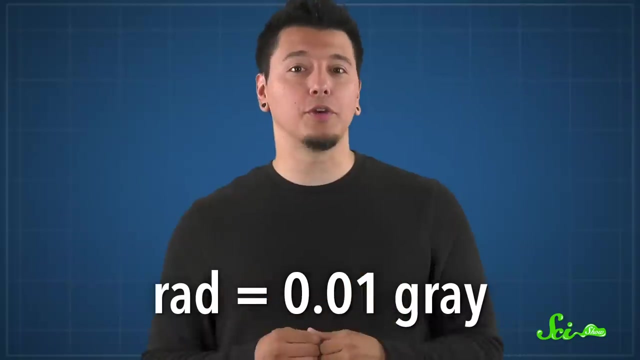 energy. For instance, a CT scan in a hospital might expose you to seven milligrays, or seven thousandths of a gray. Some people still use the rad, a historical unit now equivalent to 0.01 gray, But whether you're talking rads or grays, there's an additional complication. 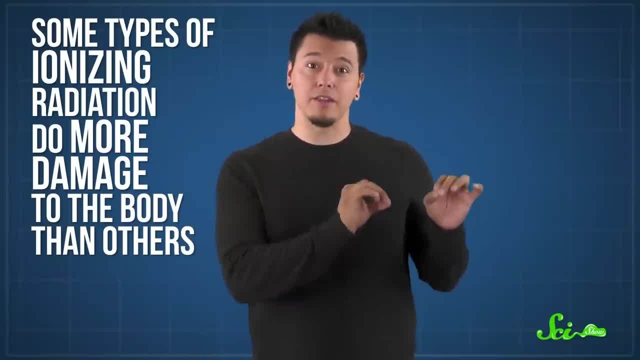 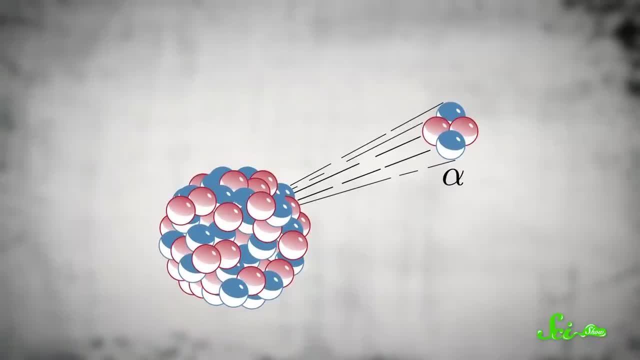 Some types of ionizing radiation do more damage to the body than others, So the same amount of grays can do different amounts of damage depending on the type of ionizing radiation. There are lots of types of ionizing radiation, but the three main ones are called alpha. 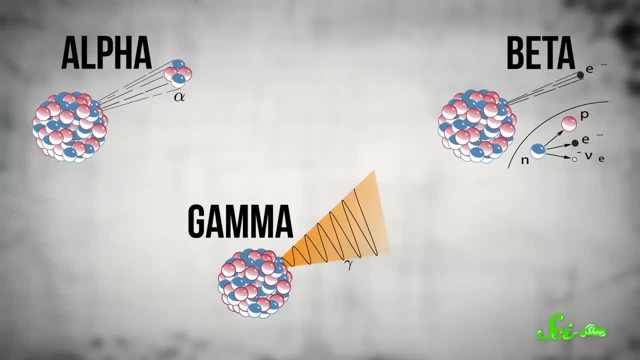 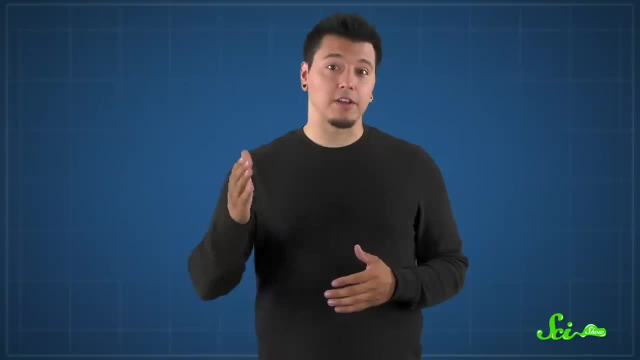 beta and gamma Each refers to a different type of particle ejected during nuclear decay. Alpha particles are the heaviest, slowest and most easily stopped, while gamma particles are the lightest, fastest and hardest to contain. And that's what finally brings us to the sievert. 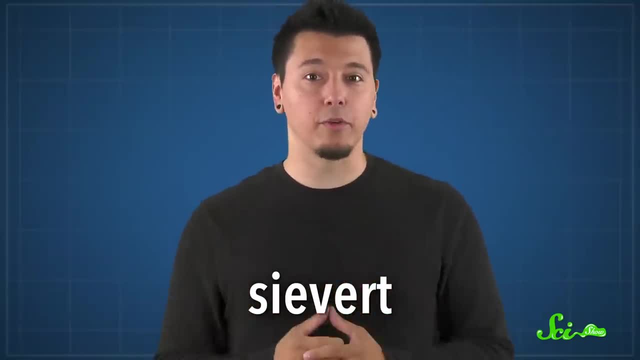 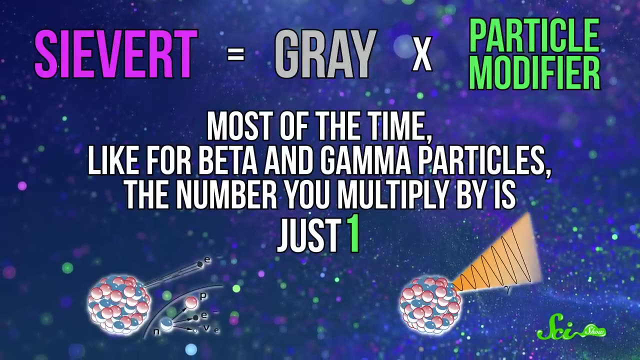 It modifies the gray to account for the different health risks associated with these particles. To get sieverts, you multiply grays by a number specific to each type of radiation. Most of the time, Like gamma particles, the number you multiply by is just one. 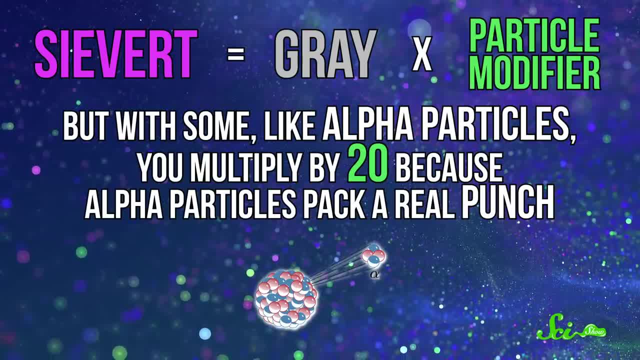 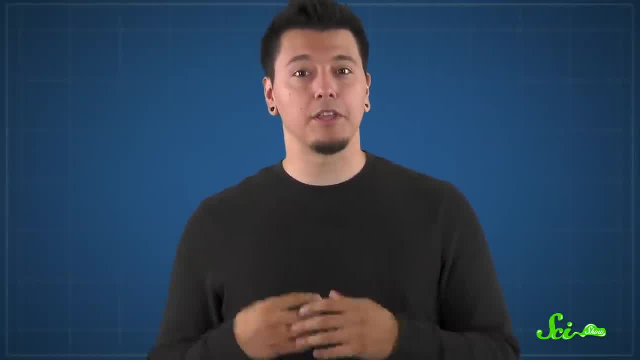 But with some, like alpha particles, you multiply by twenty, because alpha particles pack a real punch. And that twenty number isn't arbitrary. It's chosen based on the latest, constantly updated research into the effects of radiation on human health. In that way, the sievert is a unit for human convenience. 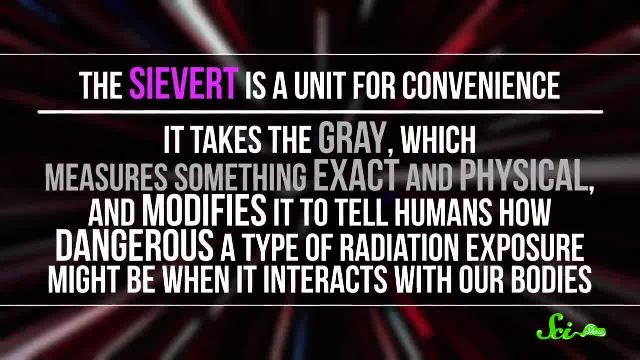 It takes the gray, which measures something exact and physical, and modifies it to tell humans how dangerous a type of radiation exposure might be when it interacts with our bodies. You also may have heard people talk about REMs when discussing the gray. It's a very common type of radiation exposure. 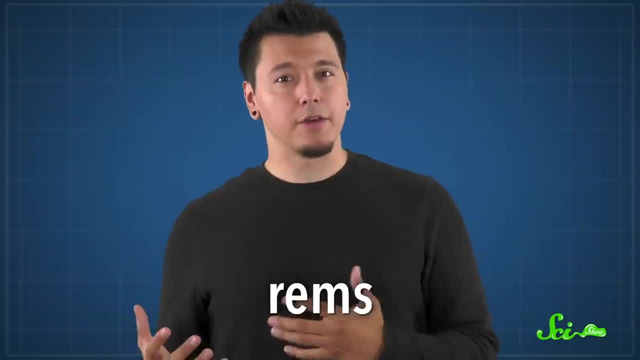 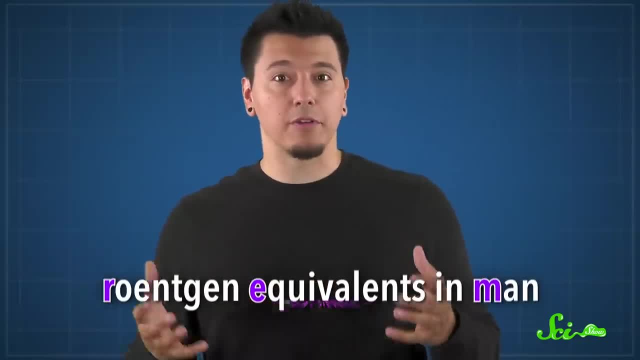 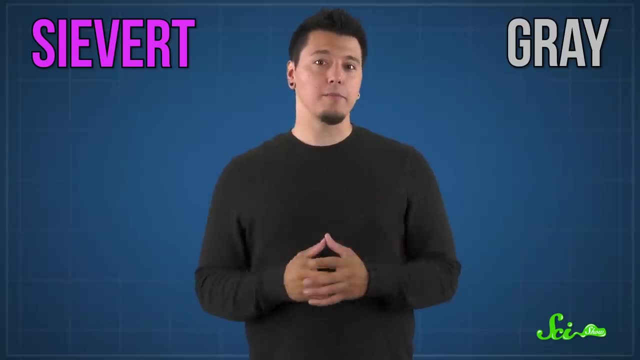 REMS is short for Roentgen Equivalence in Man. One REM is now defined to be 0.01 sieverts, But really the sievert and the gray are the only units you need to remember to understand the overall impact of radiation exposure and make informed decisions about how you travel, receive healthcare and generally live your life. Because the truth is, there are a lot of sources of radiation, including natural ones, and everyone is constantly exposed to some of it. On average, people are exposed to a few millisieverts per second. 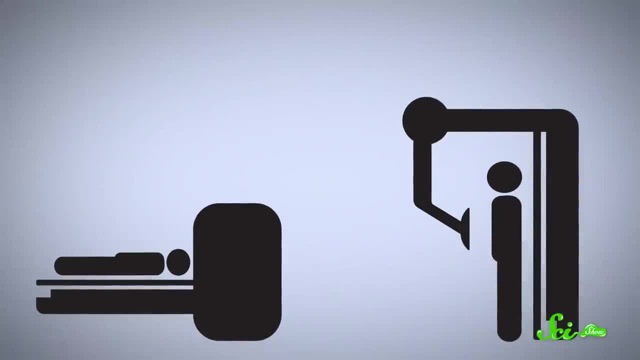 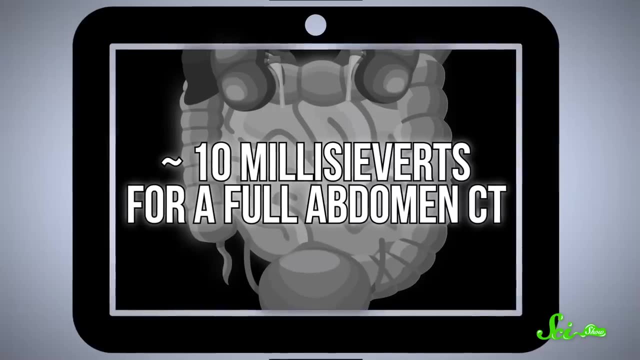 The amount from medical scans varies depending on the size of the scan and the duration in the machine: from less than 0.01 millisieverts for a quick joint X-ray to about 10 millisieverts for a full-abdomen CT. 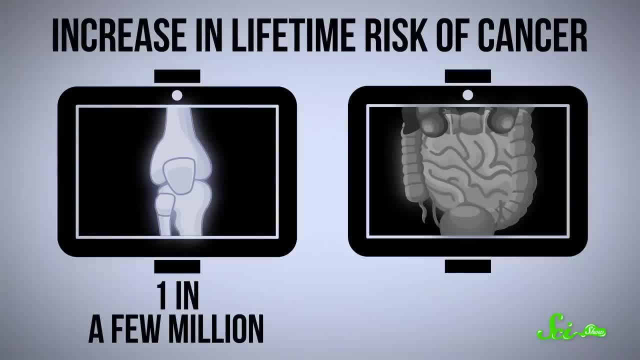 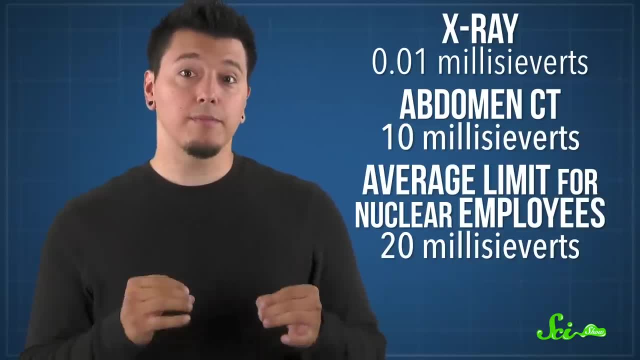 These raise your lifetime risk of cancer by 1 in a few million to 1 in 2,000, respectively. And to put all that in perspective, the allowed limit for the average nuclear industry employee is 20 millisieverts per year. 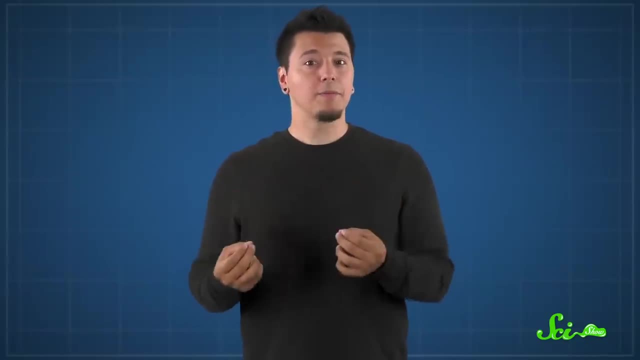 The point is, while radiation exposure can be bad, it's also something that happens to us every day, And once you understand the lingo used to describe radiation, that fact doesn't seem so scary. Thanks for watching this episode of SciShow, and a special thank you to our channel members.